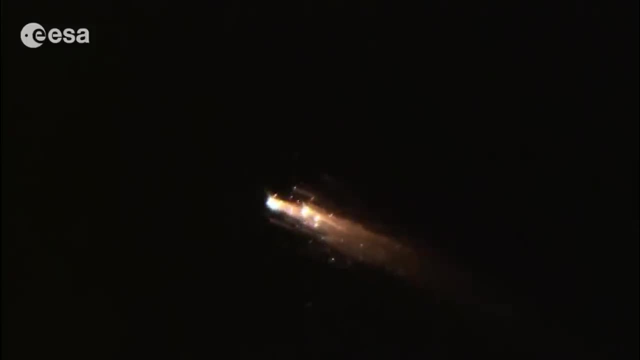 going into the spacecraft. It goes into the atmosphere instead, which is why we get those wonderful glowing re-entry trails. Spacecraft are designed to absorb as little of that heat as possible to avoid cooking the interior and the sensitive hardware inside A spacecraft might. 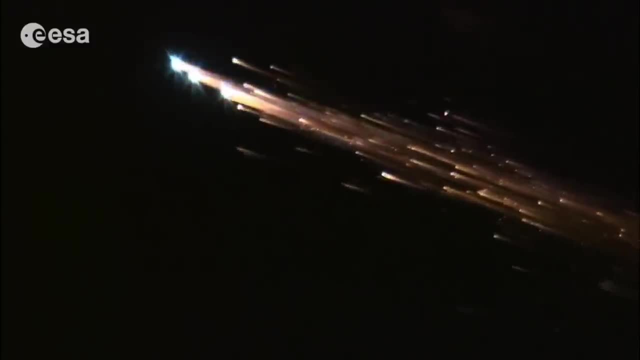 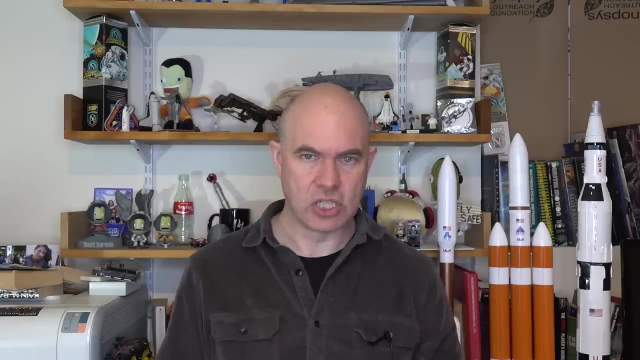 absorb, say, one to five percent of the total kinetic energy in the form of heat. The science for this really got going in the 1950s, as they were developing missiles and they were developing thermal technology. The scientists involved came up with analytical equations which did a pretty 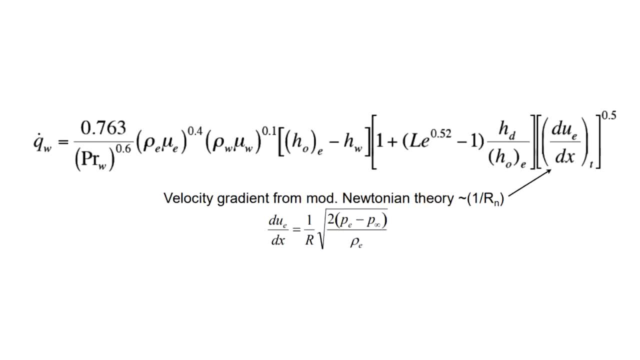 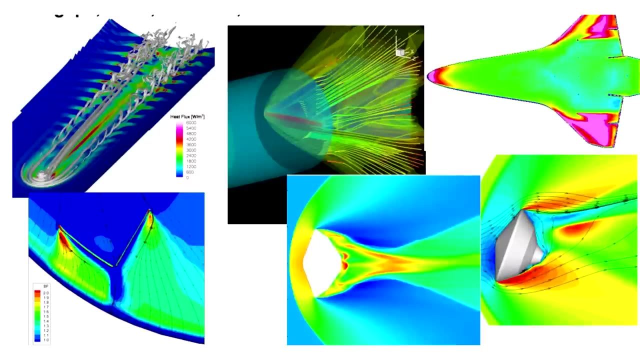 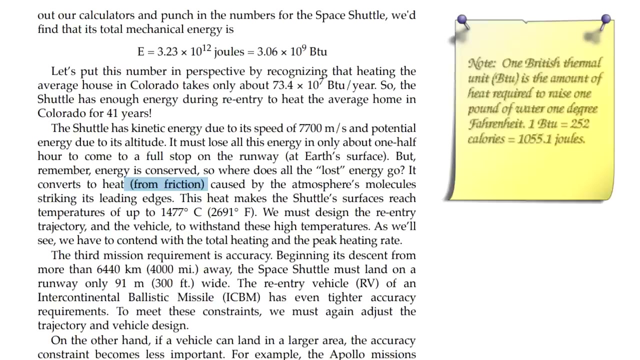 good job of modeling the heat flow, But it's such a deep problem that doing a high-resolution modeling of a modern vehicle with a modern simulation would challenge even the most powerful supercomputers available to us. Many sources state that friction with the atmosphere is the mechanism which leads to atmospheric heating, And while this is true for aircraft, 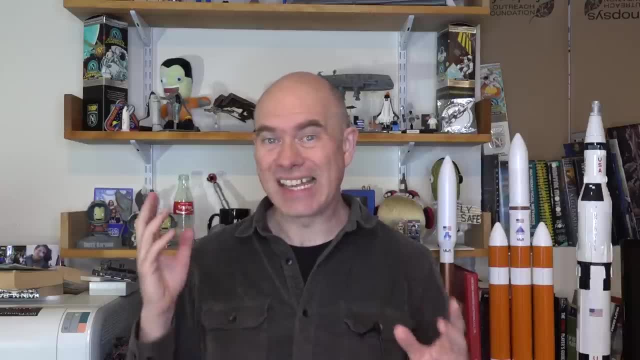 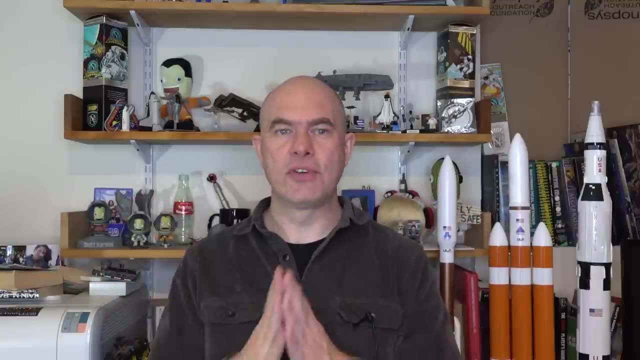 moving at supersonic speed. it's not true for aircraft moving at supersonic speed. For spacecraft moving at hypersonic speeds it's not the case. A completely different mechanism is involved. When a capsule moves through the atmosphere at hypersonic speeds, the atmosphere 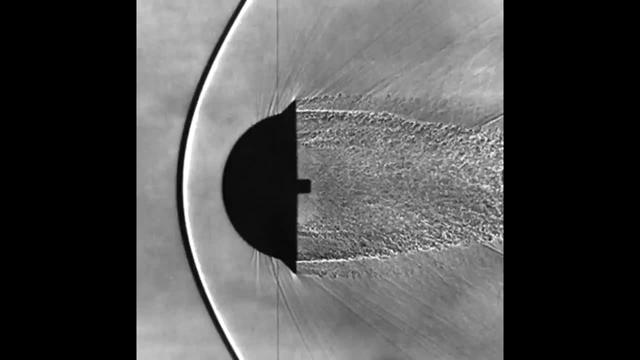 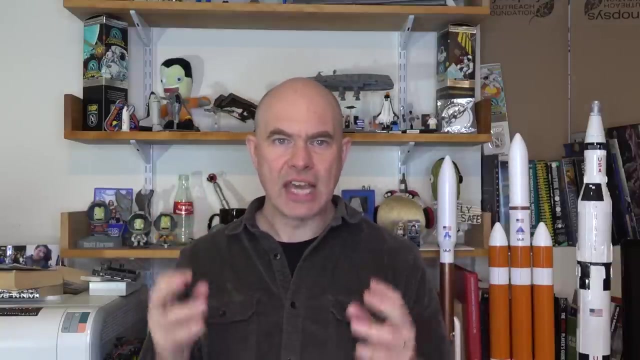 cannot get out of the way fast enough and a shockwave forms, where the velocity of the incoming air rapidly changes to match that of the vehicle, And this results in extremely high pressures and, by extension, temperatures. This shockwave forms a short distance from the body surface and it's 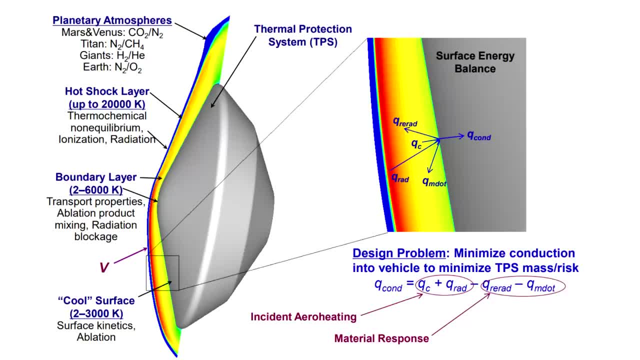 where most of the heat is going to be. So if we're going to be able to move the spacecraft to the top of the air, it's going to be at a distance of about one meter from the air surface. In this cross section, you can see that the boundary layer is significantly cooler than 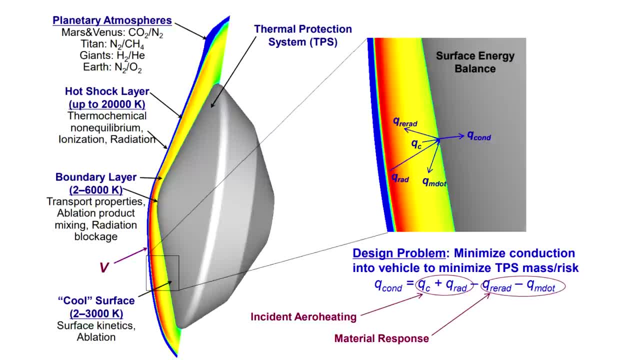 the shockwave, which is of course, a great thing for the surface of the vehicle, reducing the temperature that it's directly exposed to. So it's desirable to keep the shockwave as far away from the body as possible. Now, those analytical solutions that the Buffins 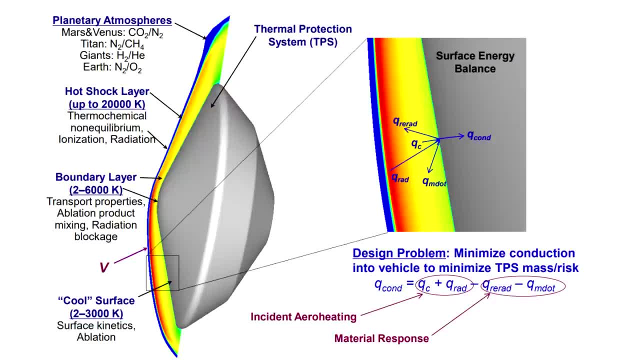 came up with in the 1950s. they showed that for a spherical body the distance to the superheated shock front is roughly proportional to the maximum heat. That's why the shockwave is so close to the surface. So if we're going to be able to move the aircraft, it's going. 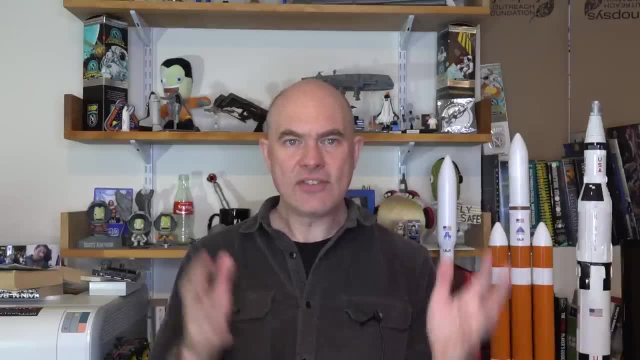 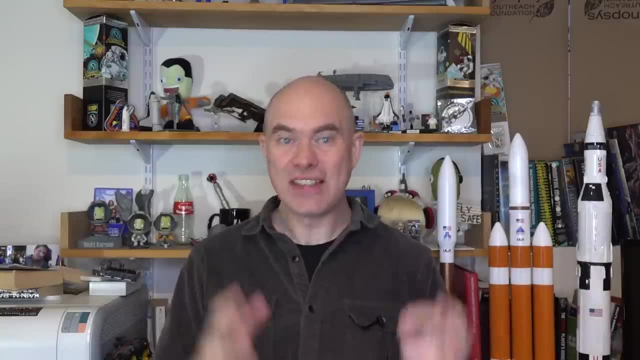 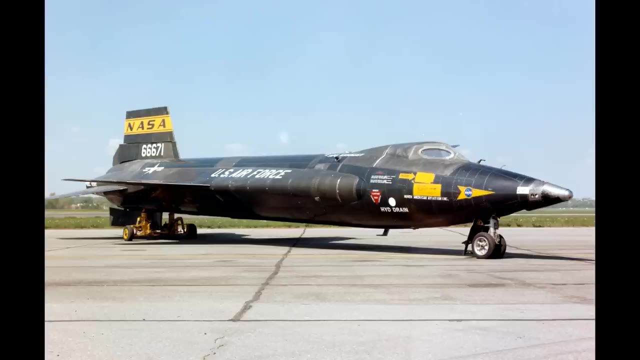 roughly proportional to the radius of the sphere, And this is generally true of any surface. The less it curves, the more it pushes the shockwave away from the surface, And this is why space planes favor blunt shapes. Compare the sharp edges of the X-15 and the SR-71, with the blunt nose of 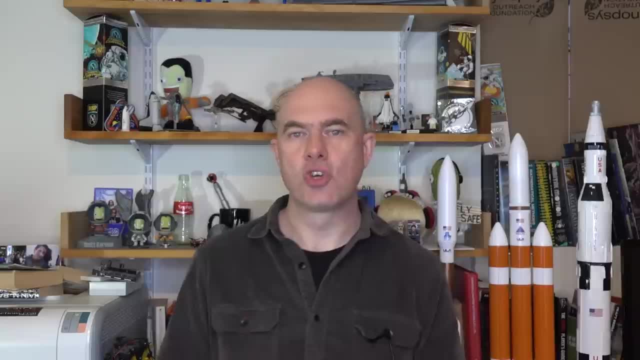 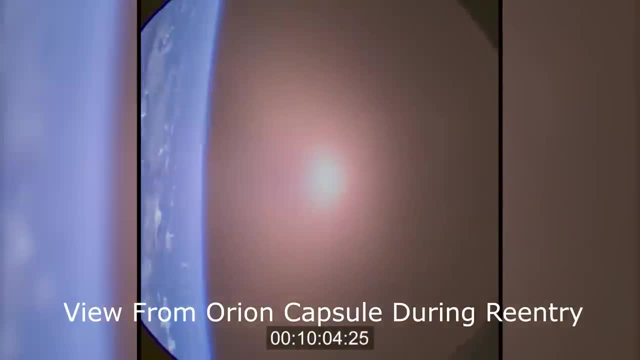 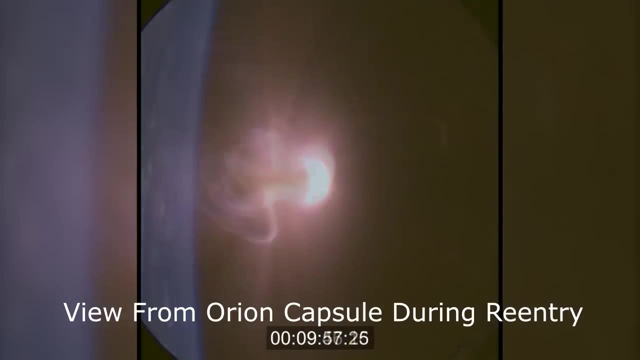 the space shuttle. The temperatures and pressures inside the shock front are easily high enough to cause the atmosphere to ionize and disassociate into its atomic species, making this atmosphere glow with the heat. This hot plasma emits significant quantities of thermal radiation which will heat the surface, And this hot plasma will actually flow around the entire vehicle. 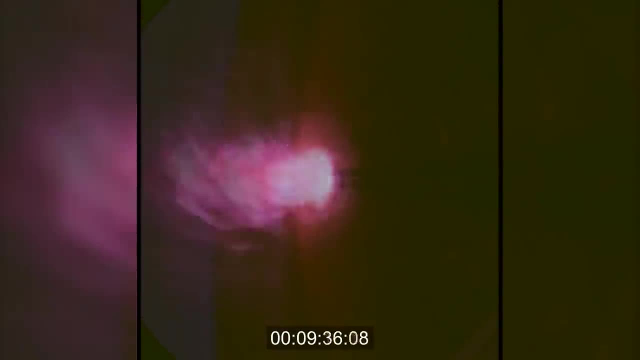 and the heat from this will actually heat the backside of the vehicle as well, And this means that there's different heating regimes on both sides of the spacecraft. On the front, a lot of the heat is coming from the contact, so you will want to actually emit as much heat as possible, So that's why the bottom of the 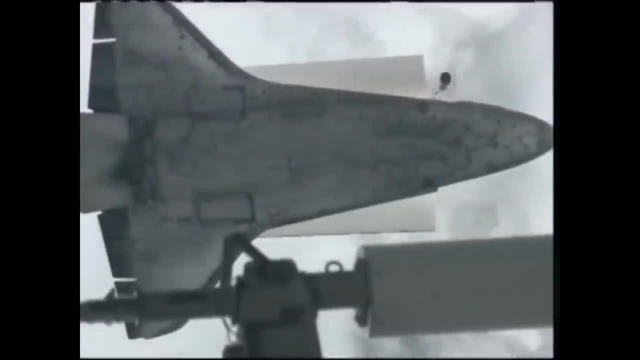 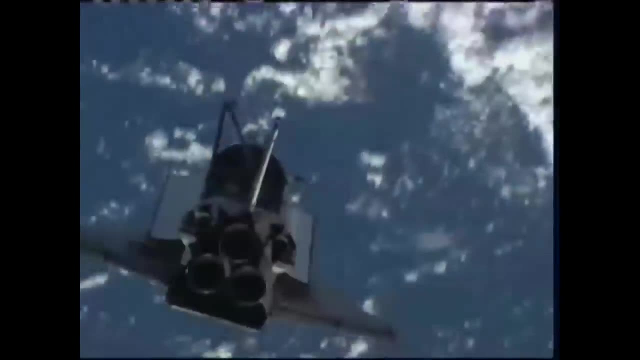 space shuttle was black to maximize emission of heat, whereas the top, well, that is only getting heated by the thermal radiation from the plasma re-radiating onto it. And that's why the top of the space shuttle was white to maximize the amount of heat that was reflected away. Now, as you go to, 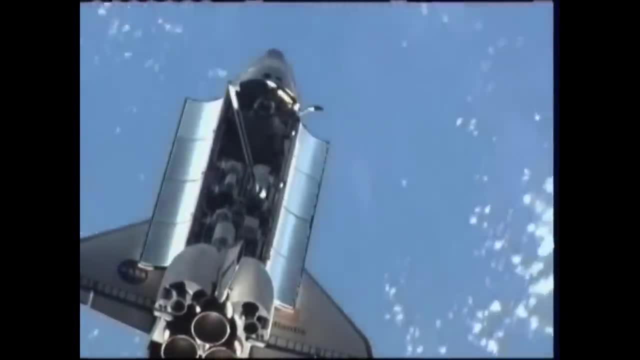 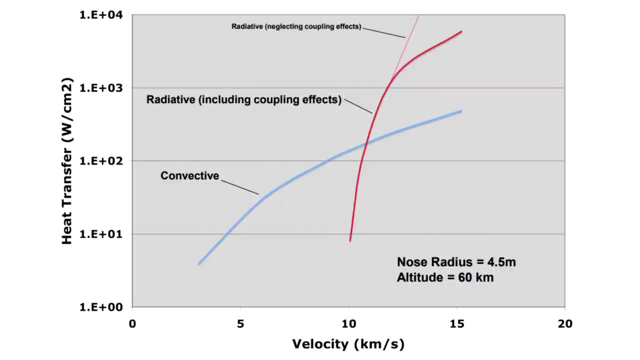 higher entry speeds, such as returning from the moon or from interplanetary space, the thermal radiation from this glowing plasma inside the shockwave actually becomes an even more efficient way of heating the surface, so that, instead of being dominated by the convection, the radiation 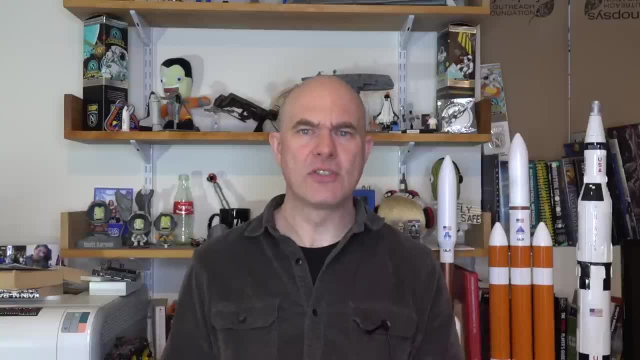 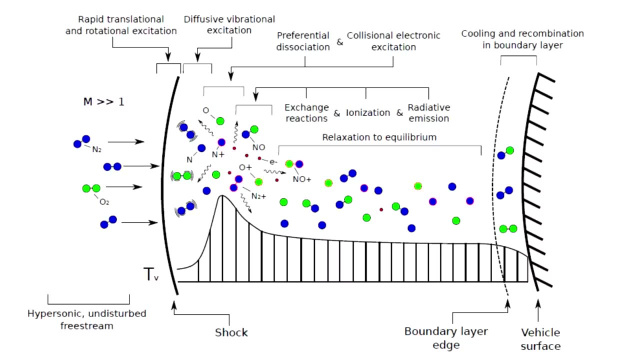 becomes more important. Moreover, those disassociated atoms and ions are, of course, chemically reactive and they will undergo reactions with each other as they flow towards the spacecraft, or they can actually have reactions on the surface of the spacecraft, with the surface acting as a catalyst. 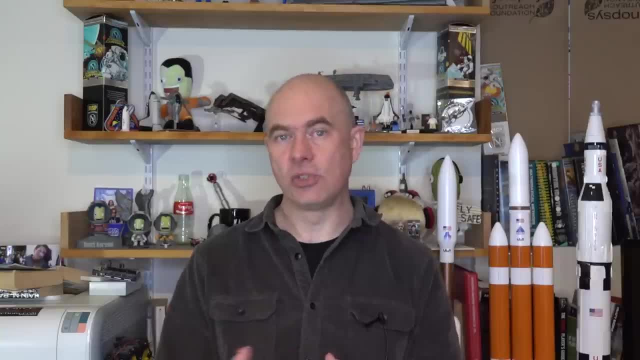 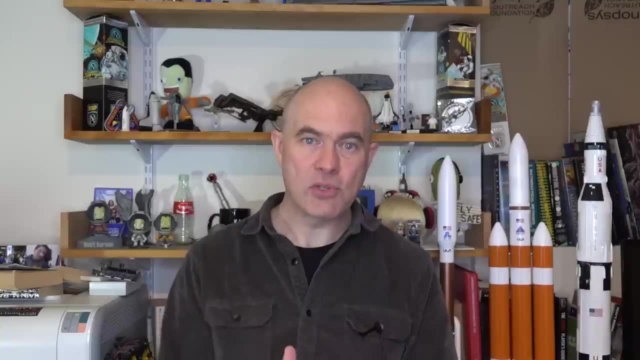 In some cases, they can chemically attack the heat shield and say, oxidize it, And this is important right The, you know, atmosphere that you're flying through. the chemistry of the atmosphere needs to be taken account of when you're designing the heat shield, A heat shield. 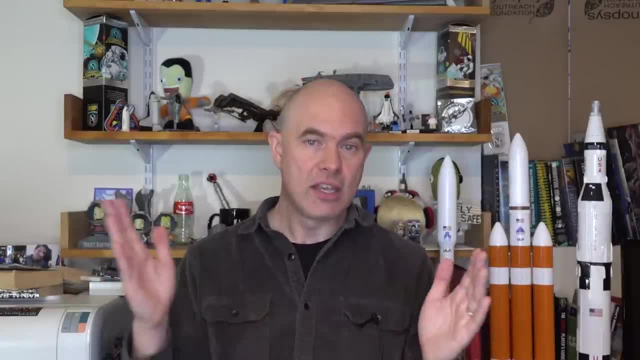 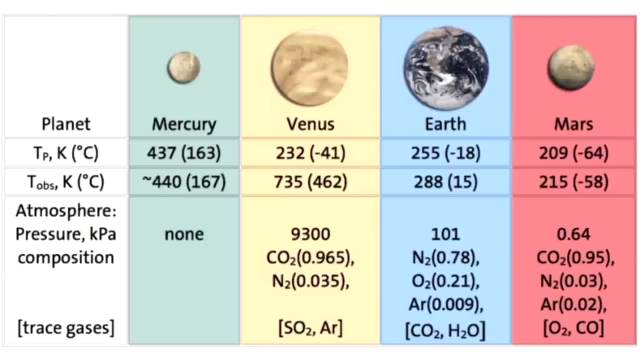 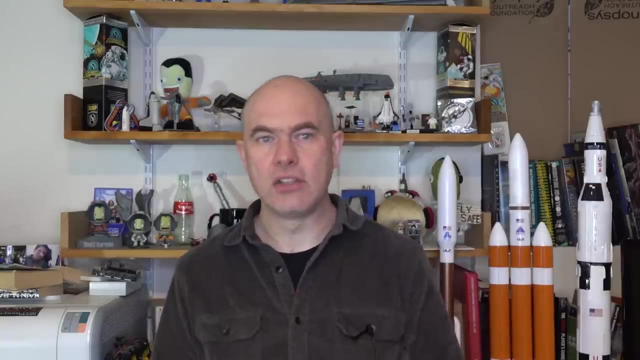 may be designed, say, for Mars or Venus with carbon dioxide-dominated atmospheres, and it might not work as well in the oxygen-nitrogen atmosphere of the Earth. So yeah, heat shields or thermal radiation Protection systems. they cover a whole range of technologies and approaches to the problem. 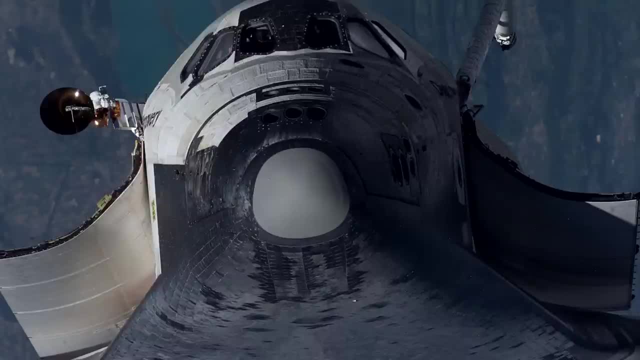 Probably the easiest design to understand is the space shuttle's heat shield, with its patchwork of tiles, thermal blankets and reinforced carbon-carbon components. The materials were able to handle high temperatures on the surface and had very low thermal conductivity. So what they did? 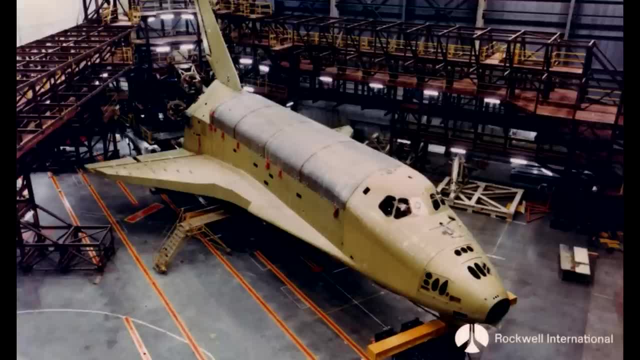 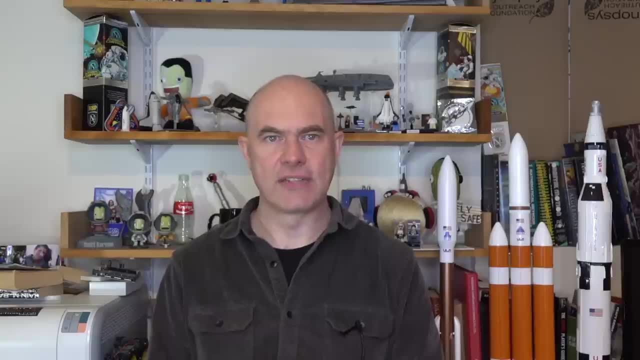 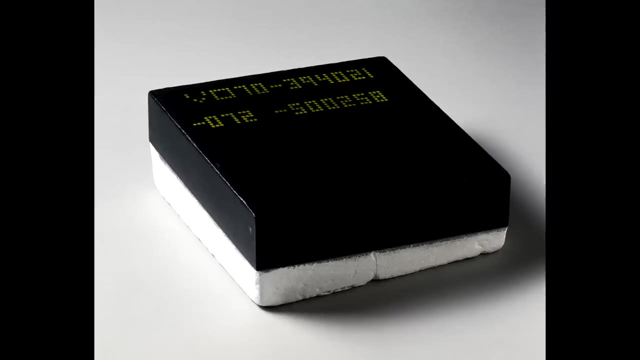 was they stopped the heat conducting inwards towards the aluminium skin and structure. The tiles were a low-density foam or sponge made with silica glass fibers and sealed with a glass coating. The result is a material able to handle skin temperatures of about 1200 Celsius, while 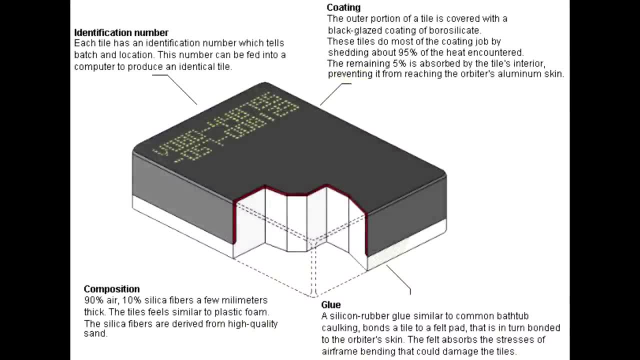 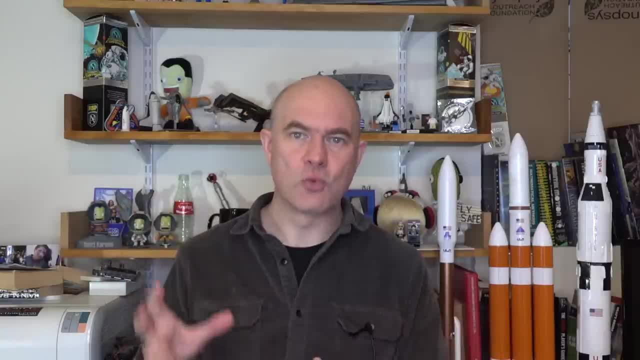 minimizing the thermal conduction and also being light enough for space flight. The thermal conduction is incredibly low on these, so low that there's a famous demonstration where they placed one of these tiles inside a furnace and heated it up to be red hot and they were able to. 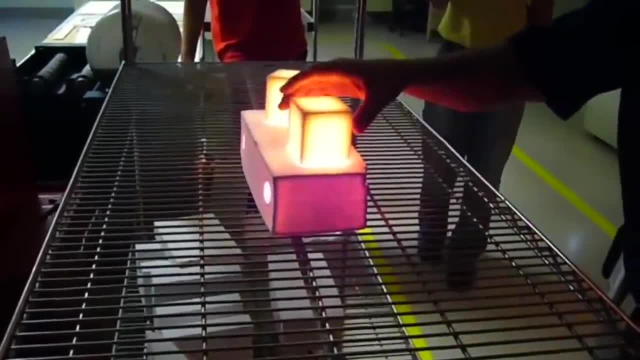 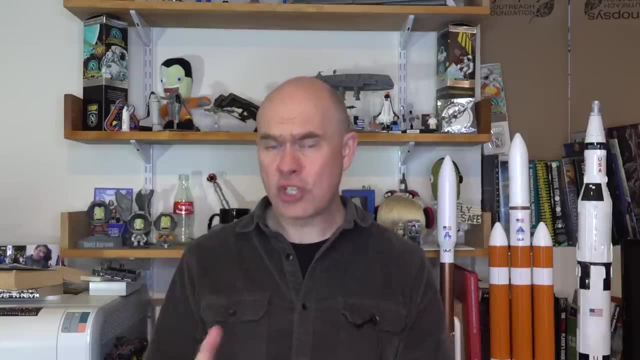 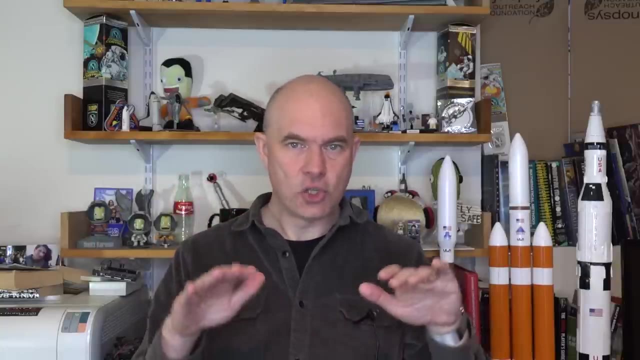 and they would then take it out and carefully hold it in their hands while it was still glowing hot. but they were also extremely fragile. you could crush them with your bare hands. please don't do that. if they're red hot, you will burn yourself, and also they had a tendency to pop off. 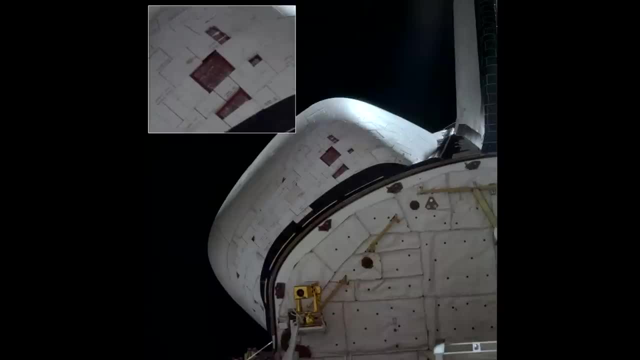 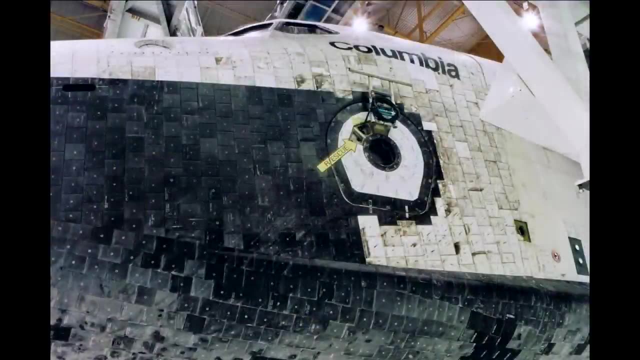 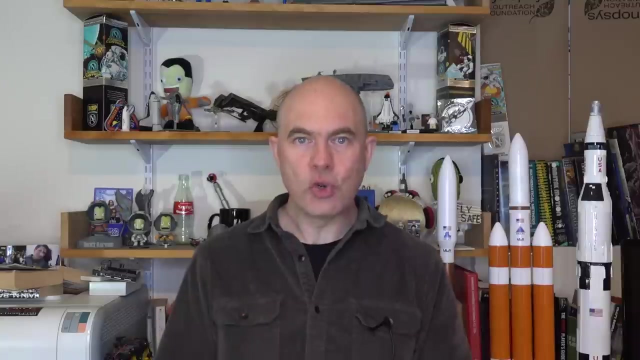 the structure of the spacecraft as the as it flexed from aerodynamic forces. now, early on in the shuttles program, the the low temperature tiles on the top were largely replaced by thermal blankets, which were more flexible and would be less likely to detach during atmospheric entry. the tiles would accept the thermal energy and they would slowly conduct the heat inwards towards the aluminium skin. the tile thickness varied across the vehicle to account for the differing heat loads. then some places they were up to like 12 centimeters thick where the flow of heat would be had. 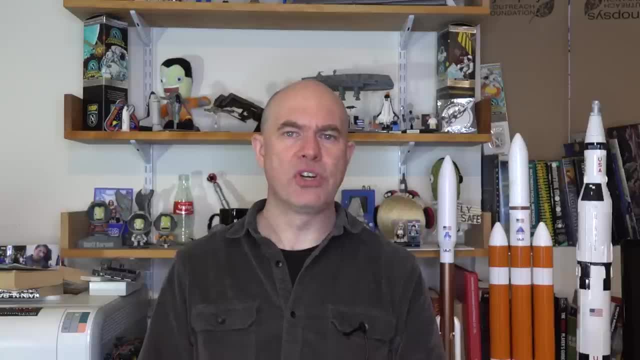 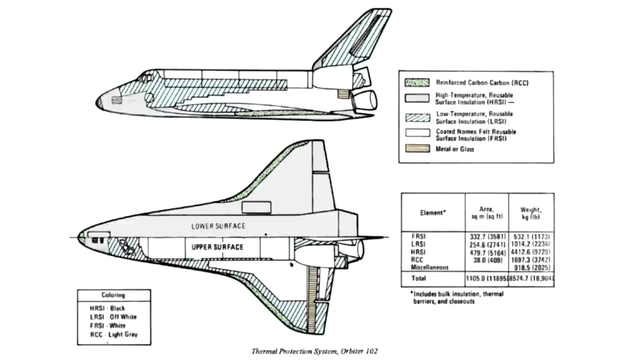 to be slowed for as long as possible, but in places where aerodynamics dictated sharper curves, like the nose and leading wing edges, the shock wave would be closer in and the heating was significantly higher still, and the glass-based tiles were simply not enough. instead, the shuttle used reinforced 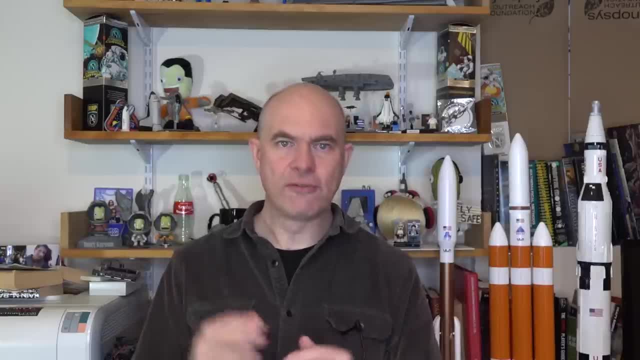 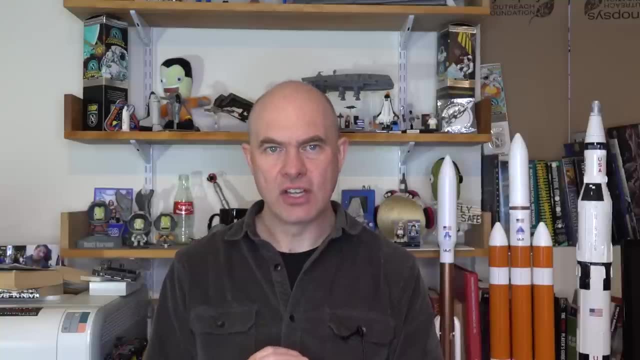 carbon-carbon, that is, graphite reinforced with carbon fiber, which is able to understand or to withstand temperatures of about 1500 Celsius, which is a very high temperature, and it was also able to handle extremely high temperatures. you might not realize it, but that pencil lead which is soft. 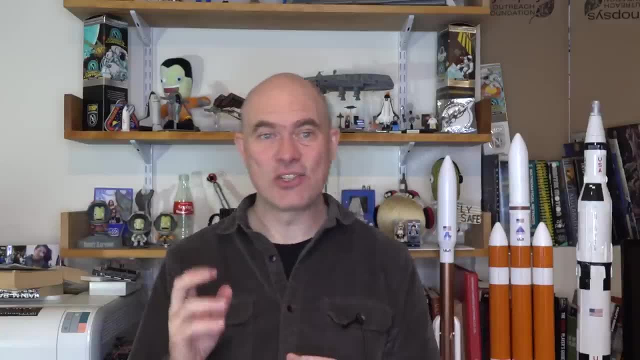 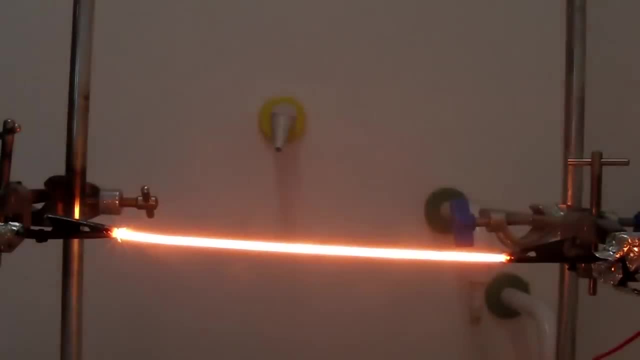 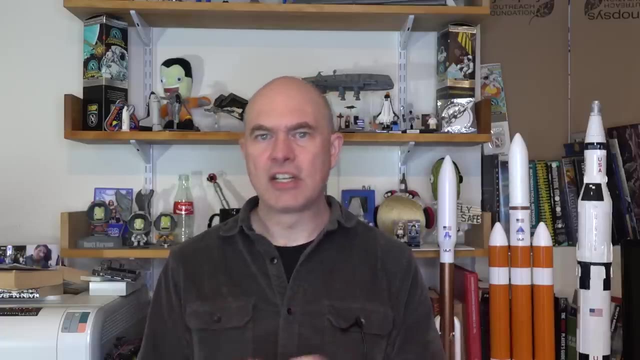 enough to write on. paper is actually able to handle extremely high temperatures. it can get as high as like 4000 Celsius, making an excellent component of heat shields. it does, however, have a tendency to oxidize when heated in an oxygen atmosphere, so the carbon-carbon components would be covered. 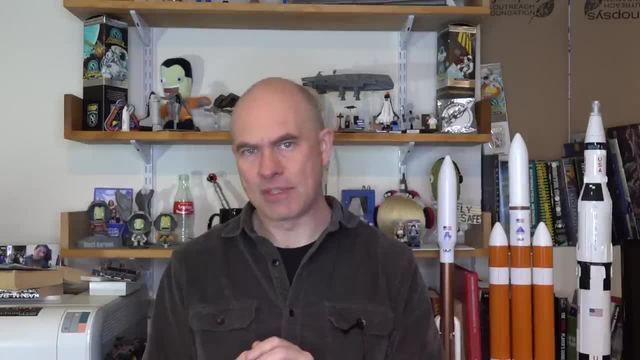 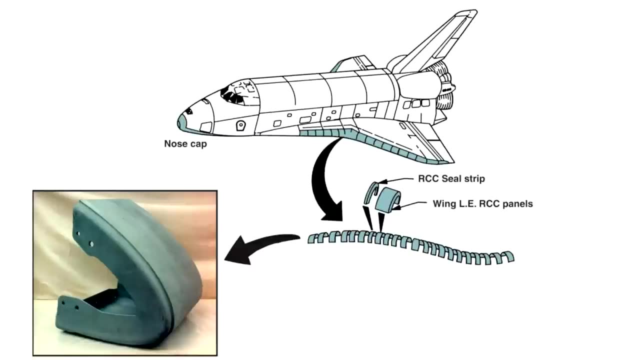 with a layer of silicon carbide to insulate it from the atmospheric oxygen. unlike the tiles, the carbon-carbon components were actually quite strong and they didn't need a structural skin beneath them to hold their shape. it was, however, a lot heavier than the tiles, which meant that they 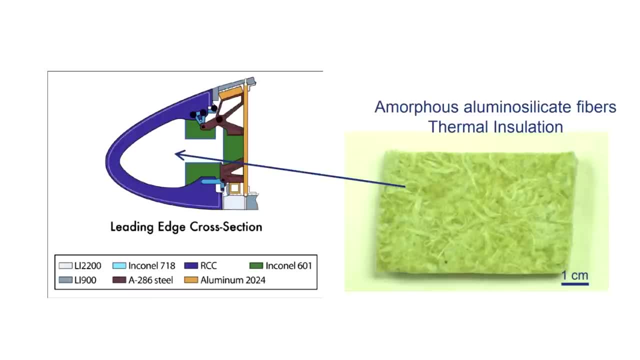 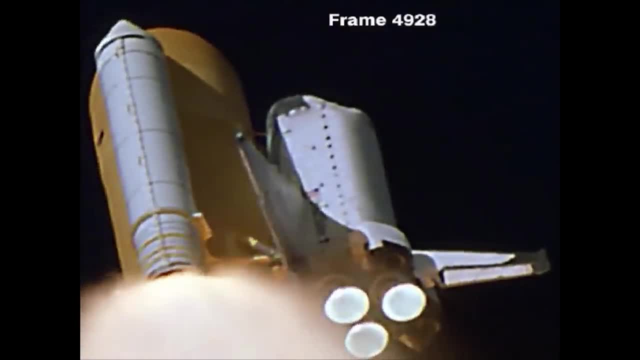 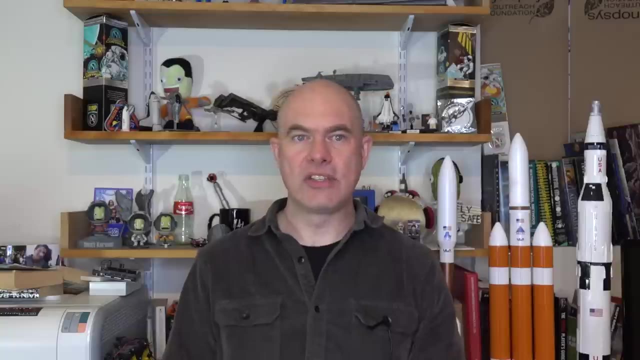 were only used in the places where it was absolutely necessary. and, yes, the carbon-carbon wing edge was strong, but it wasn't strong enough to handle the impact of a chunk of foam, which led to the loss of the shuttle columbia in 2003.. less well known is the case of sts-20. 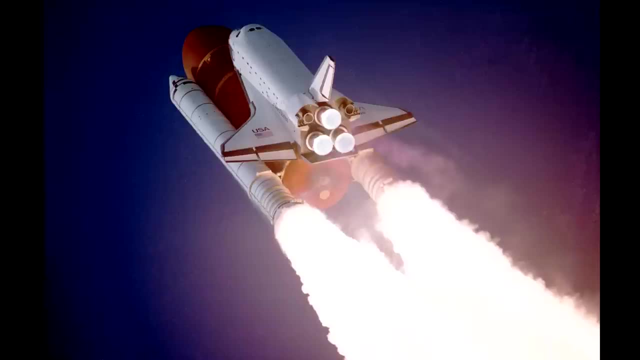 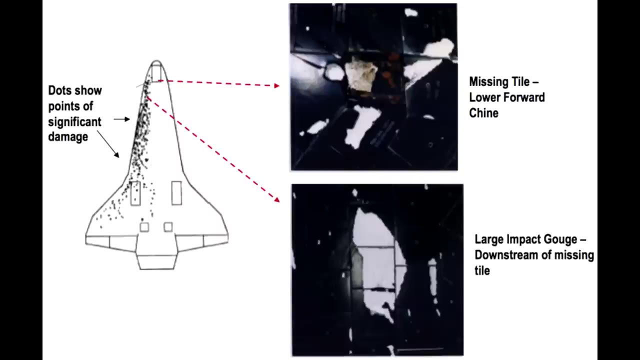 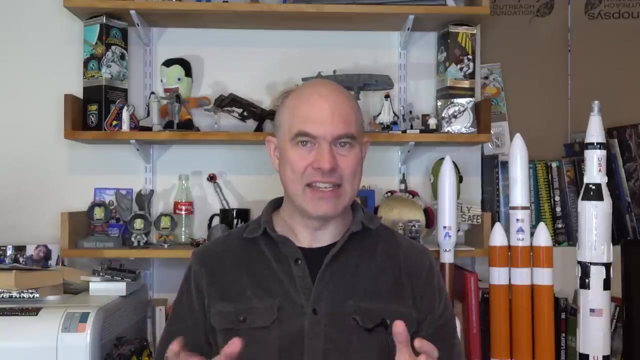 7, which was a classified mission. there was debris that was lost from the starboard booster and then it struck the spacecraft, knocking a tile loose. the crew were concerned and they wanted to get images to the engineers on the ground, but because it was a classified mission, they had to send it via an 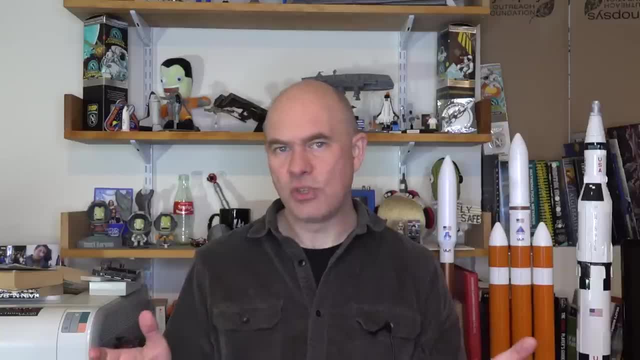 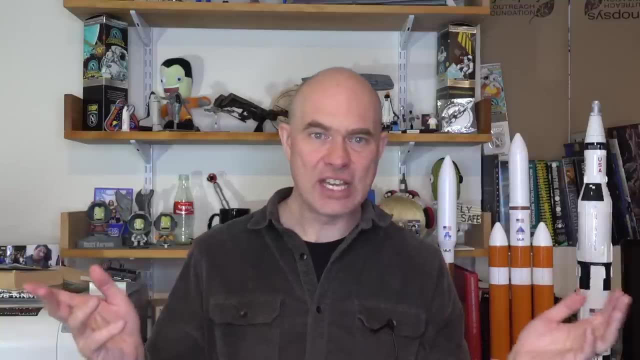 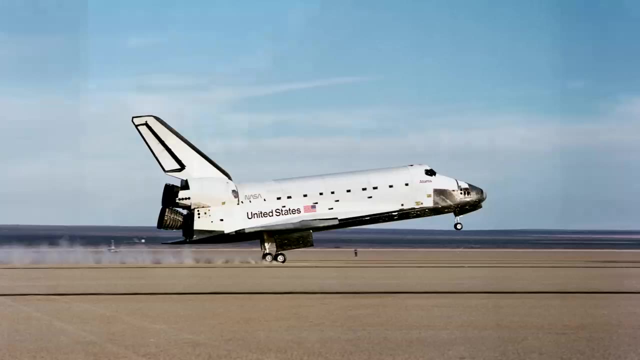 encrypted television signal and the engineers, when they looked at it they couldn't see what the astronauts were seeing and they told the astronauts they thought it was fine, it was just shadows, even with a tile missing. sts-27 landed successfully, but the damage was evident as soon as people came to the spacecraft. the survival of the vehicle is actually credited. 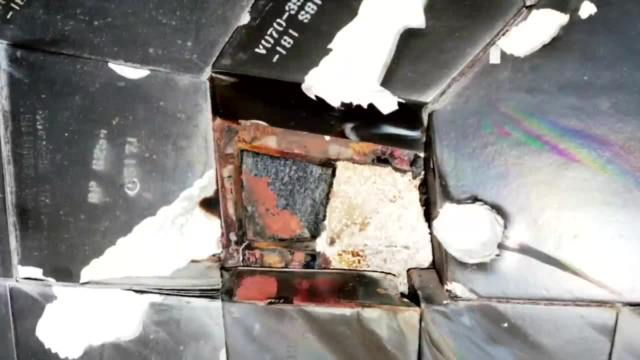 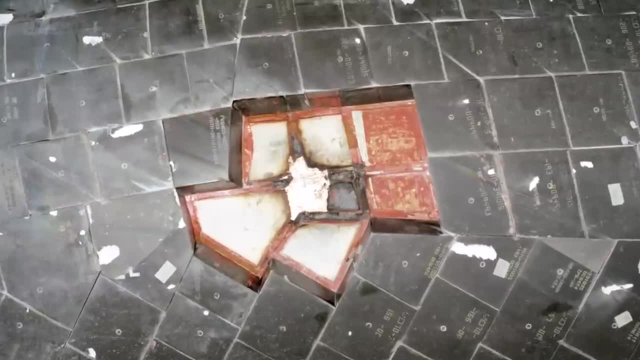 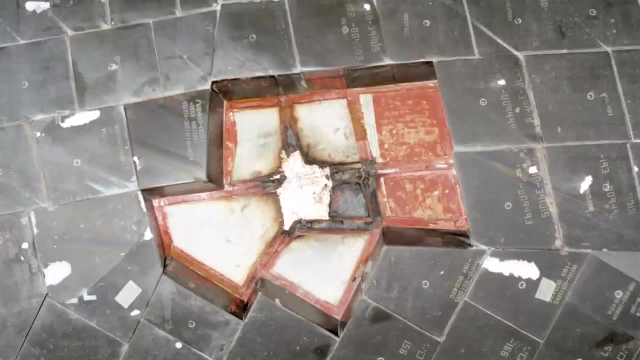 to the fact that the tile that was lost happened to sit directly under the steel mounting plate for the l-band antenna. anywhere else it would have probably burned through the aluminium skin, but the steel was able to handle the heat a whole lot better and therefore the crew survived now. 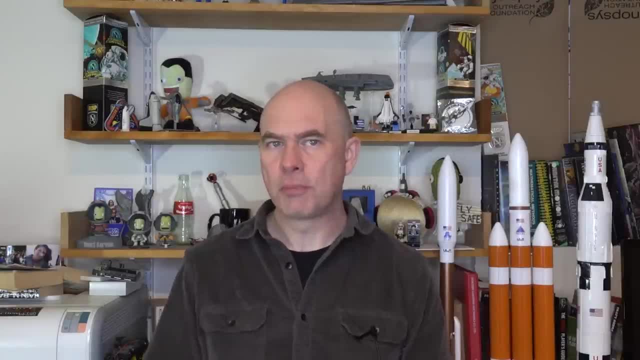 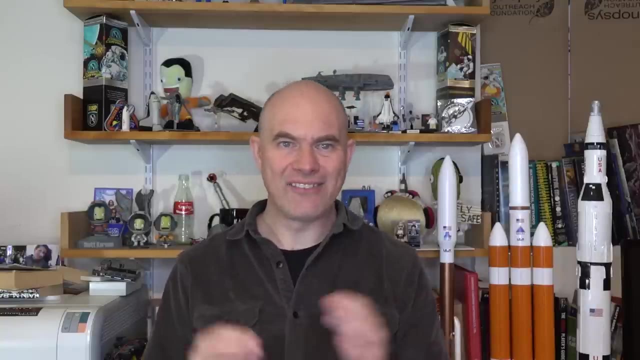 despite the problems with accidental damage, the shuttle's thermal protection system was designed the way it was because it was supposed to be reusable. while the post-flight inspection and repair was laborious, it was a lot easier than stripping and replacing the entire shield after every flight. furthermore, small defects and bumps would generate turbulence, which would mean. 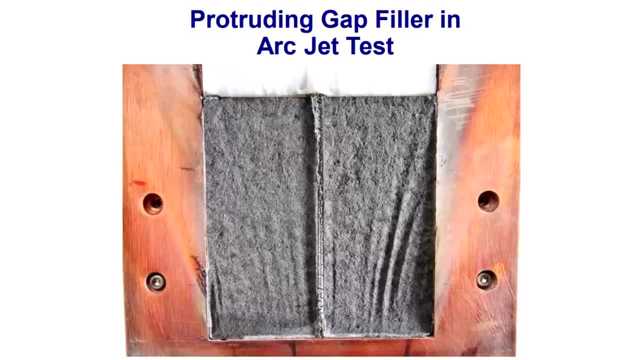 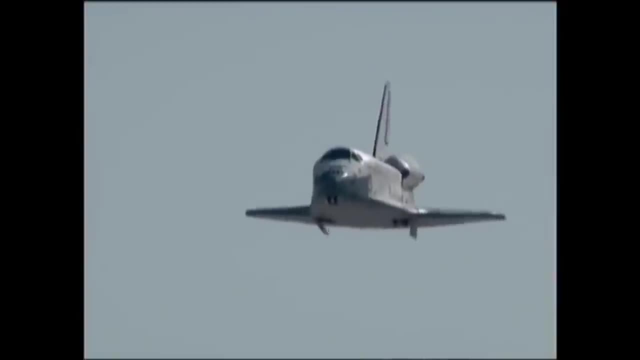 hot spots and hot spots if would wear down the shield faster in those locations. and so this third would cause what's called thermal pitting, and this could actually seriously affect the aerodynamic properties of the vehicle. and you know, the shuttle was not the greatest aircraft to begin with, so the shuttle heat shield wasn't supposed to wear down over time. 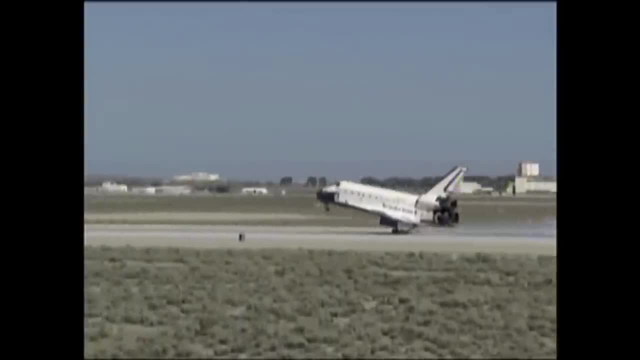 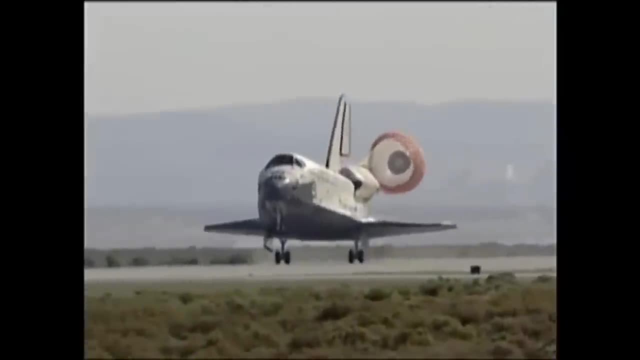 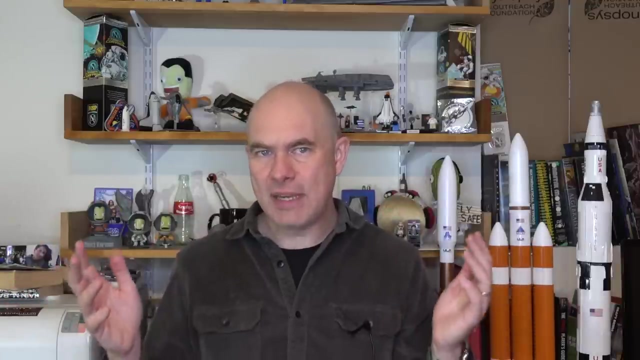 unlike the apollo capsules. yes, i know i'm going back in time here, but the heat shield and the shuttle acted like an insulator without any chemistry or any physical change, as expected. unlike the heat shields- that was you were used on basically every single other spacecraft. most space capsules use a heat shield that's designed to ablate. that is the heat causes. 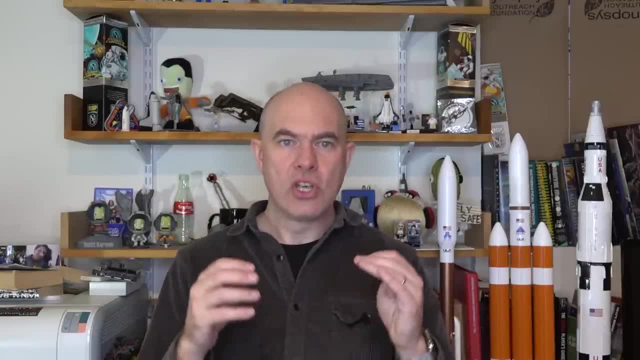 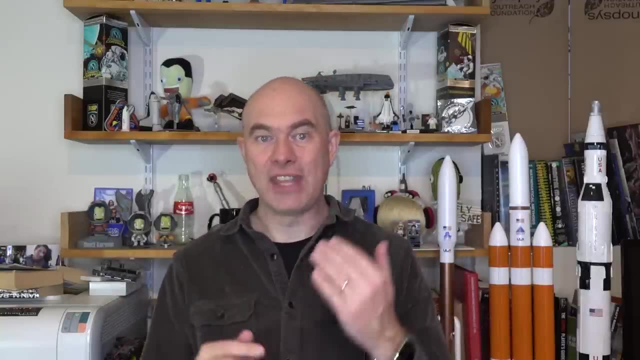 chemical and physical changes in the material which cause parts of it to evaporate away in a gas. this process actually helps in three different ways. first of all, the chemical reactions and phase changes will take heat in. secondly, the escaping gas lets the heat escape into the capsule. 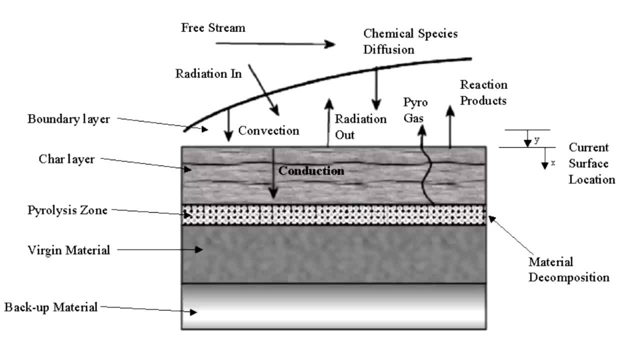 literally will carry this heat away from the spacecraft. finally, as the gas escapes, it will form a boundary layer that will protect the spacecraft. it will insulate it from the actual atmosphere. so ablation is actually a very powerful mechanism to keep the spacecraft protected from atmospheric heating. the apollo capsule heat shields had to handle return from much higher. 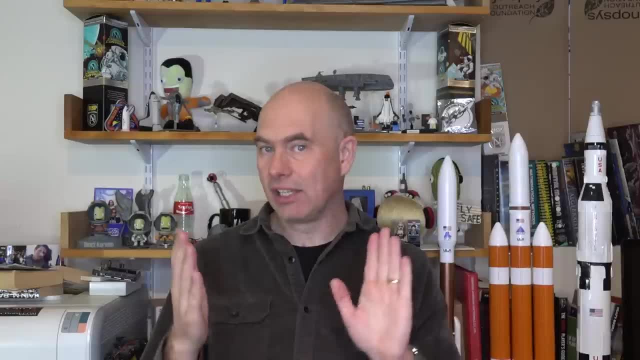 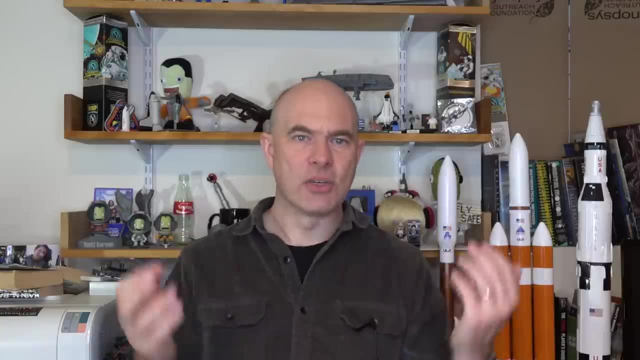 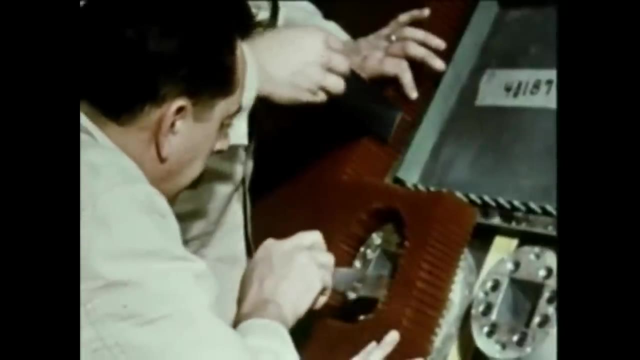 speeds than the space shuttle, but its heat shield was actually a lot thinner because it was designed instead of materials that remain intact at thousands of degrees celsius. the shield is primarily made of a plastic which can't handle more than a couple of hundred degrees. specifically, it 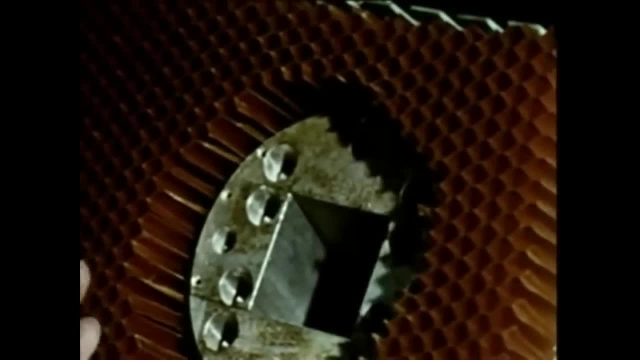 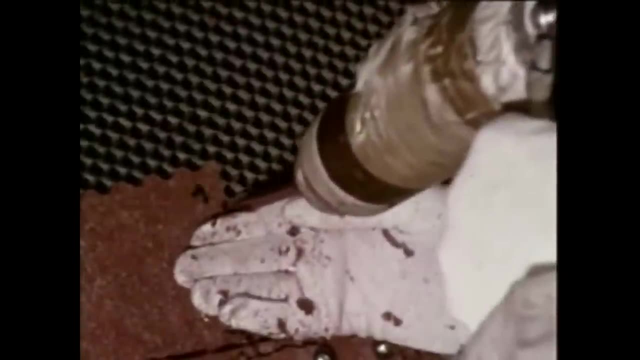 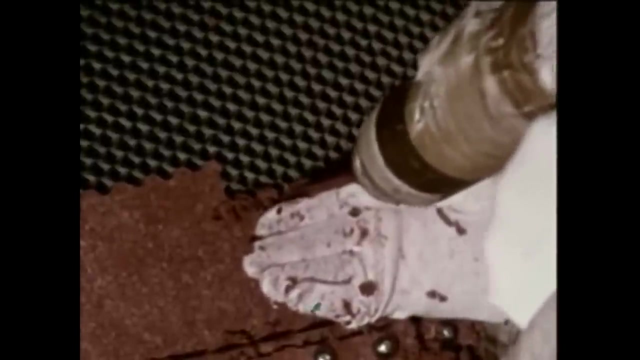 was made from a phenol formaldehyde resin, which was supported by a honeycomb structure made of fiberglass. now, manufacturing this heat shield was terribly labor intensive. after laying down the fiberglass honeycomb, a worker would have to go and inject the resin into each one of these little cells using something that looked like a cult gun. this, understandably, would. 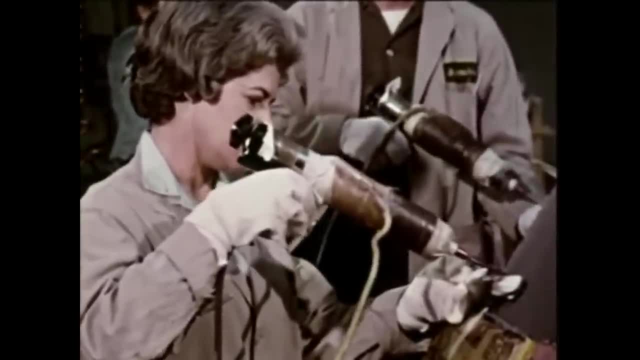 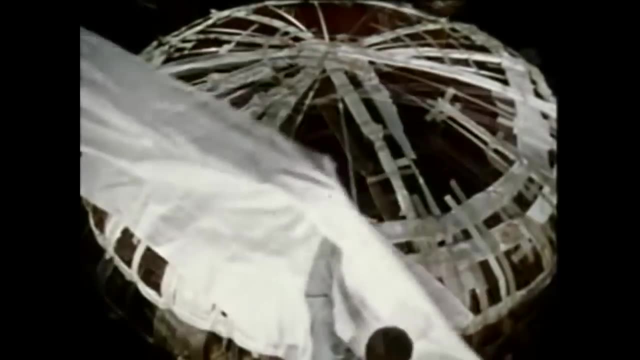 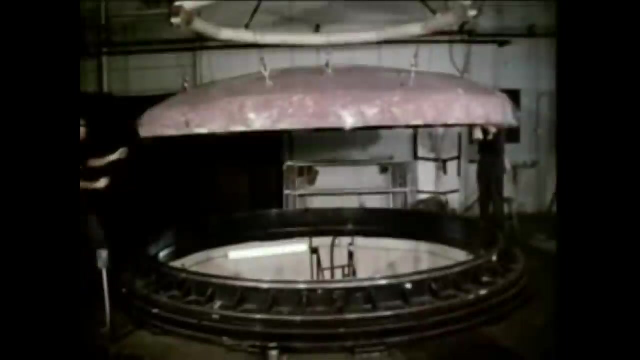 take a really long time. you might imagine that a heat shield largely made of plastics would melt and flow away, but it's actually a thermo setting plastic. that means the polymers are essentially interlinked and wound together so that, instead of melting and reforming in different 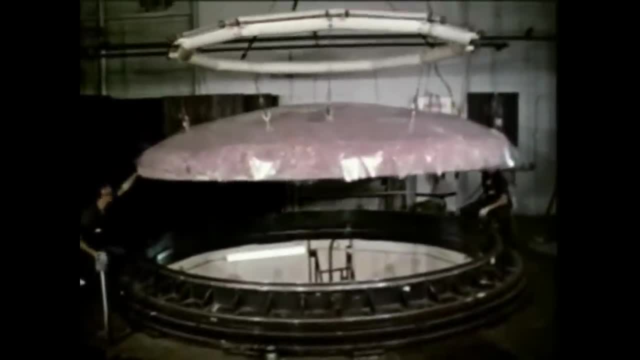 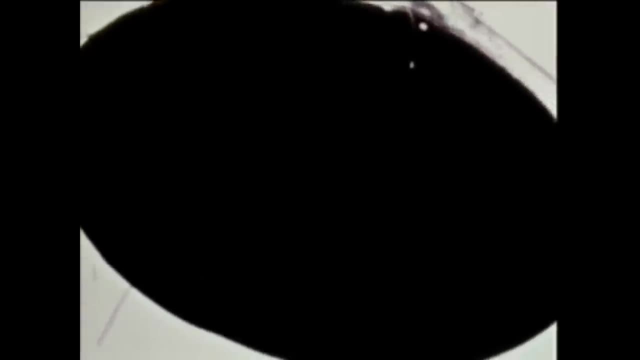 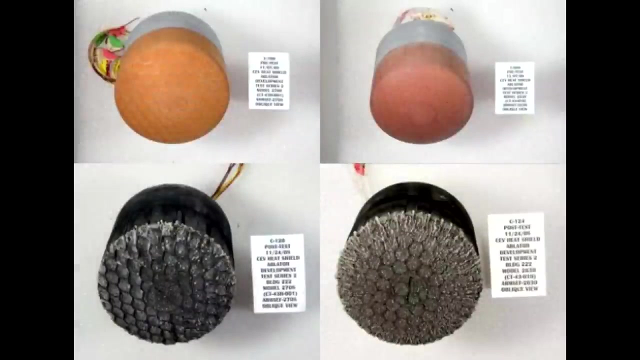 shapes, it literally just starts to break down chemically. what happens is various gases start to get evolved as it gets heated. you'll get, you know, water, methane, carbon dioxide, carbon monoxide, but what's left behind actually is a significant amount of carbon, so it literally turns black. the 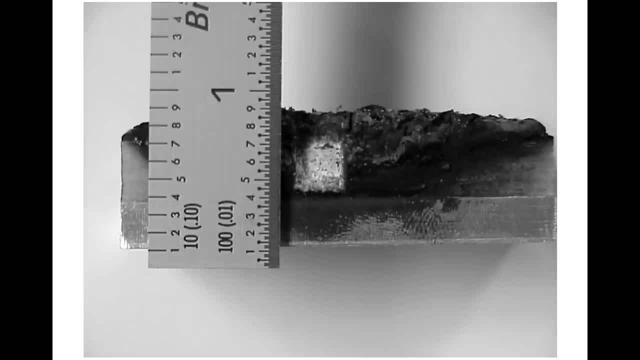 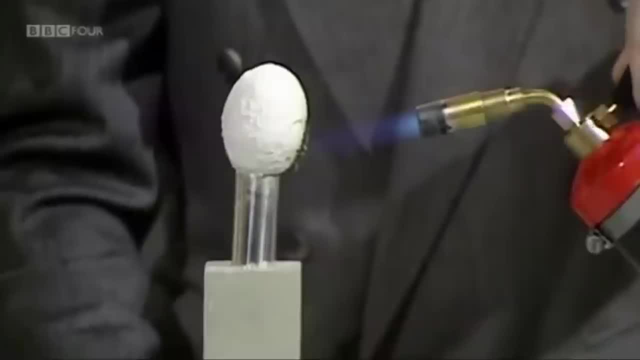 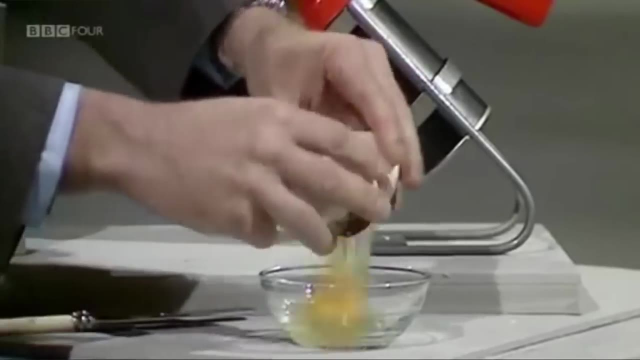 low density carbon that's left behind is actually an incredibly good insulator that will further protect the material beneath it. now, of course, some of you have mentioned starlight, which is, of course, this mysterious compound that was famously used to protect an egg from the heat of a blowtorch. this basically works in in a very similar way, as it. 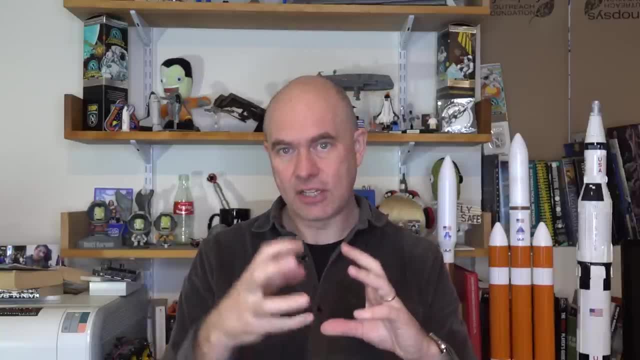 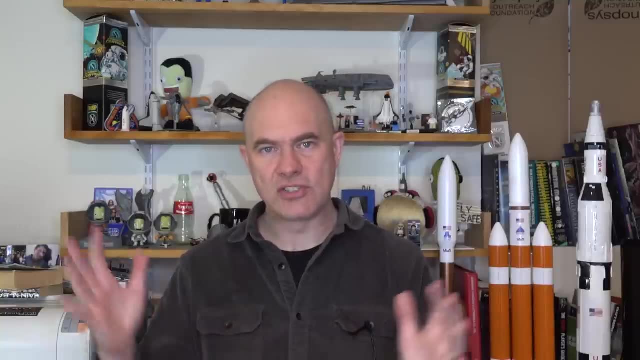 burns, it creates this thin layer or this thick layer of carbon that expands out. of course, the stuff that was used on the apollo heat shield had to be much more structurally sound, because it's flying through the atmosphere at hypersonic speeds and with the apollo heat shield 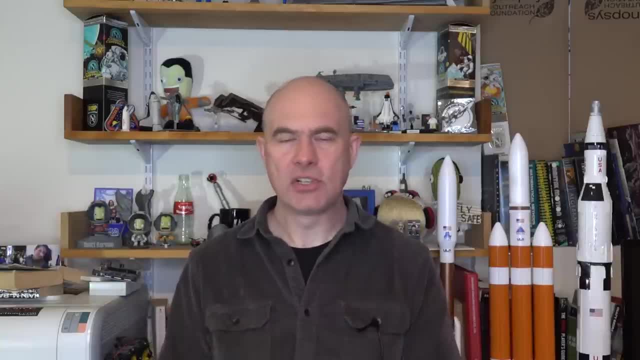 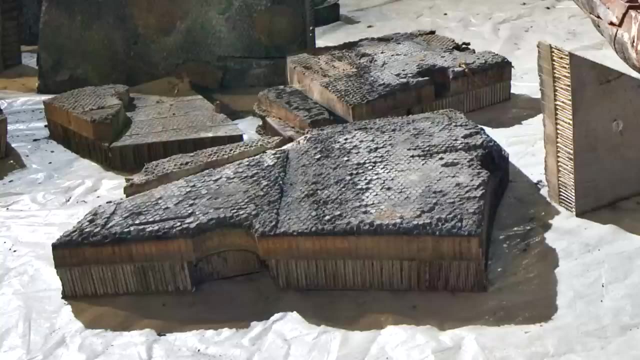 had a density of about half a gram per cubic centimeter and the char layer that would be left density to about 0.23 grams per cubic centimeter, that's less than half. about 55 of this would be the fiberglass was there and then 45 would be the carbon. that was left, a more modern version of this. 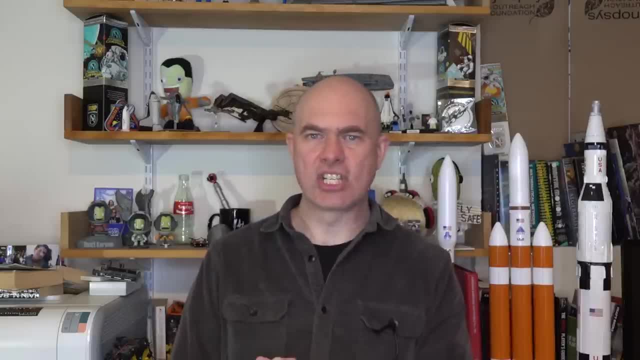 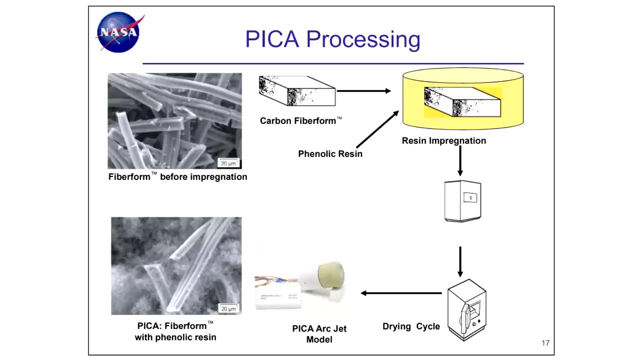 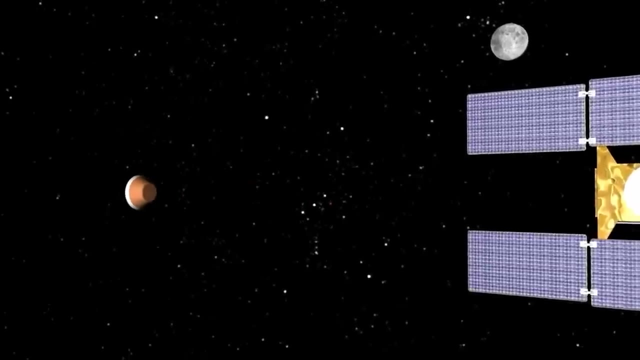 is the pica heat shield phenolic impregnated carbon ablator, where the fiberglass honeycomb is replaced by a carbon fiber sponge or foam and the resin is more or less soaked into this structure. so it's a very, very nice and very interesting and very interesting machine to work with. 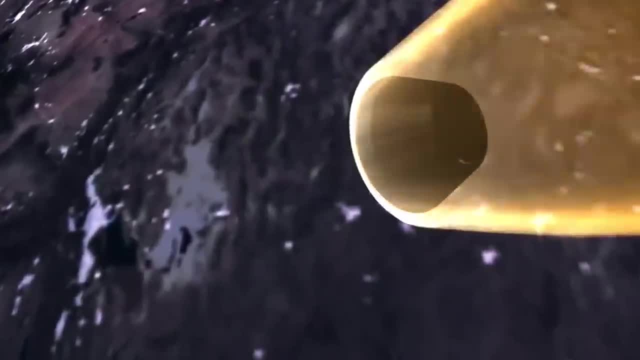 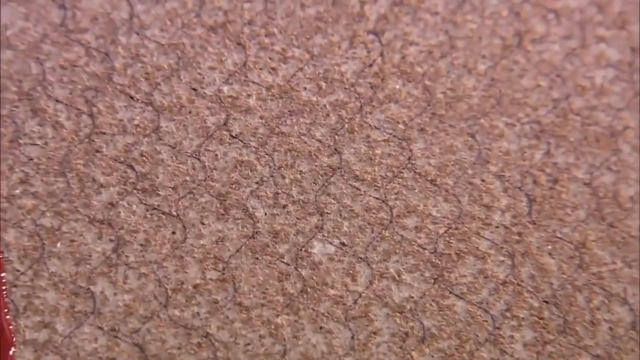 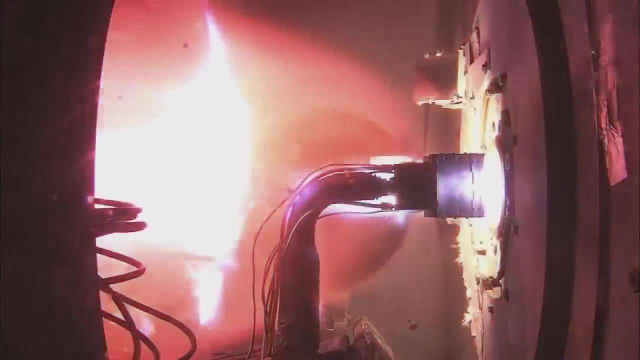 so to speak. so pica was first used for the stardust sample return capsule, which still holds the record for the fastest entry into the earth's atmosphere by any spacecraft. the spacex have taken pika and developed it further, creating something called pika x, which is largely an improvement designed. 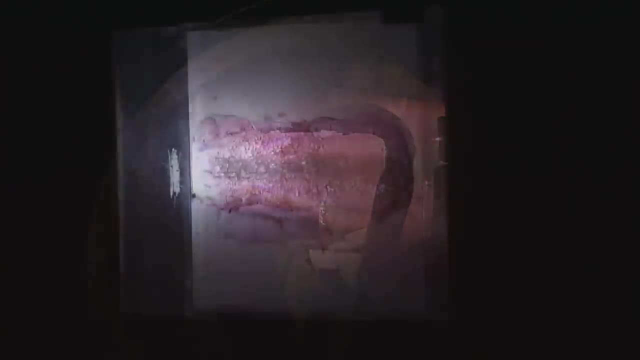 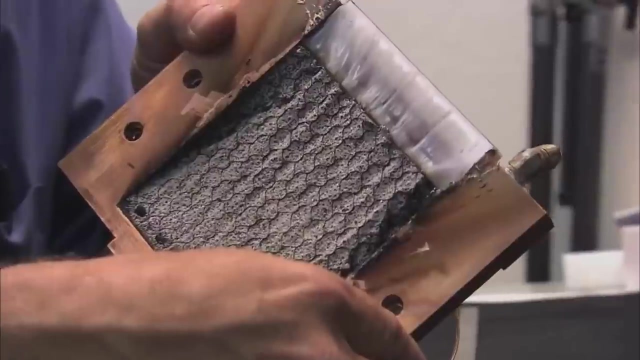 around manufacturing it more easily. it's been used on their dragon capsules, for you know, 16 launches now. the dragon capsule is the main mechanism by which the international space station returns experiments to earth. now spacex have been reusing their dragon capsules, but it's not like the space shuttle. the 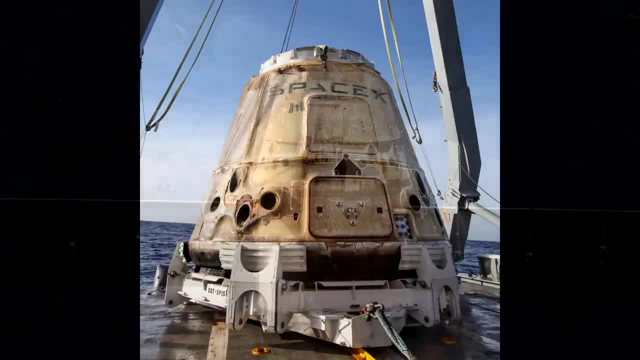 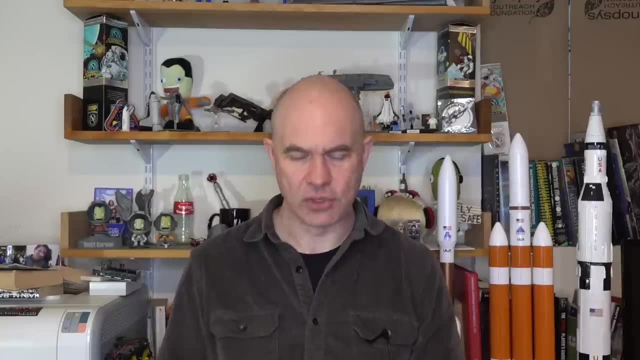 heat shield. damage is quite extensive, and to reuse it they have to literally strip off the heat shield and put a new one on. the most extreme heat shield ever used was on the galileo atmosphere probe, which flew into jupiter's atmosphere at a healthy clip of 48 kilometers per second. 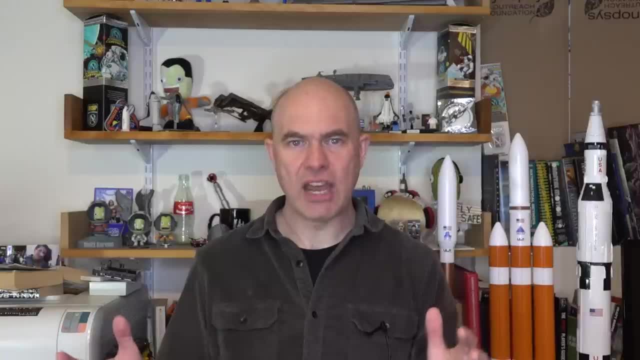 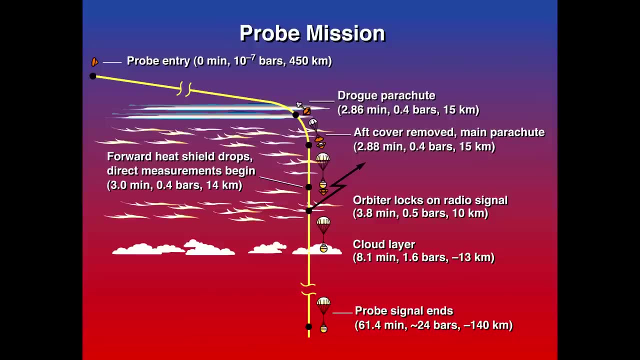 the spacecraft was only about 300 kilograms, and half of that full 150 kilograms was on the heat shield. during re-entry it slowed at rates approaching 230 g's. it had hit temperatures of something like 16 000 degrees celsius, and by the time it slowed down and was able to deploy its 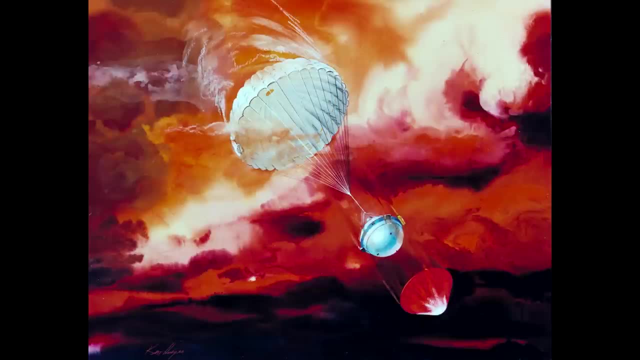 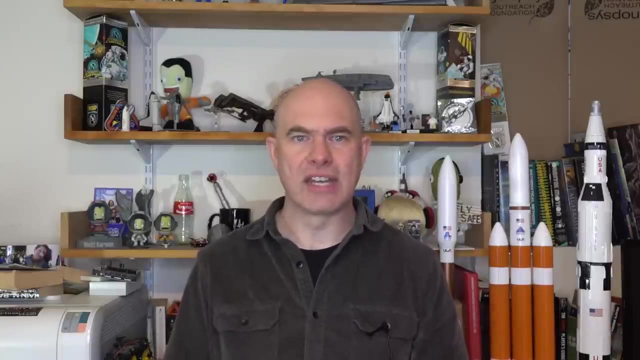 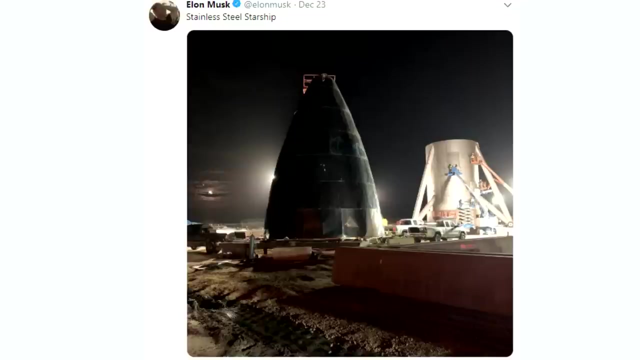 parachute. it had fully ablated away 82 kilograms- more than half of the heat shield. but looking to the future, spacex are reportedly working on an actively cooled heat shield for their starship vehicle. according to elon's twitter feed, the spacecraft will use a shiny stainless steel. 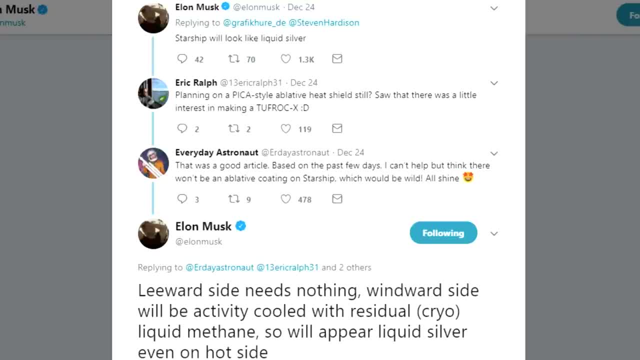 structure with liquid methane from the fuel tanks circulating just under the surface to keep the skin cool during re-entry. only one half of the surface would need to be cooled in this way. the leeward side would still get heating from the plasma, but uh, that could be a little bit more.